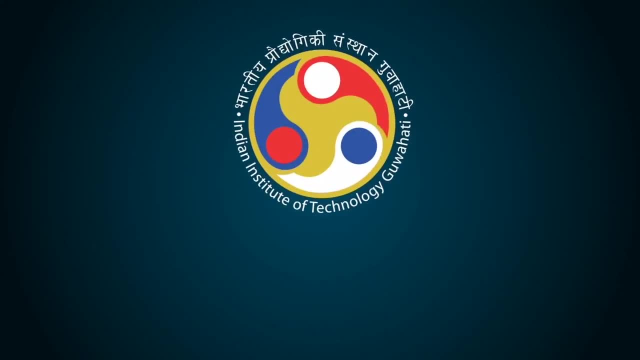 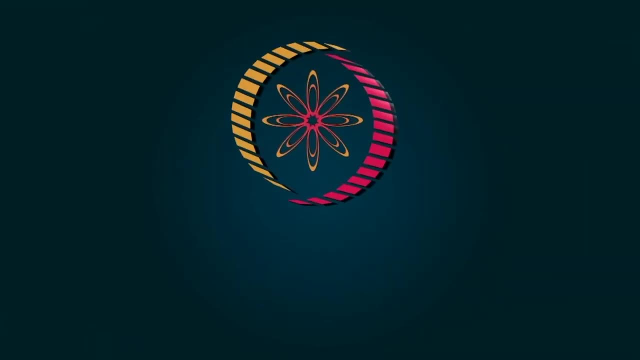 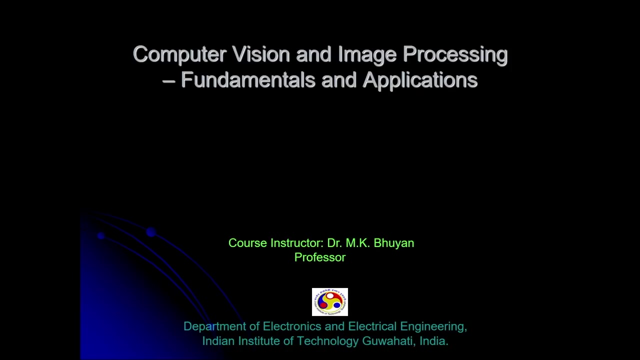 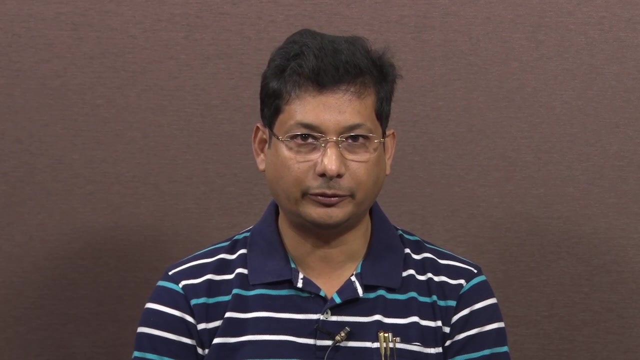 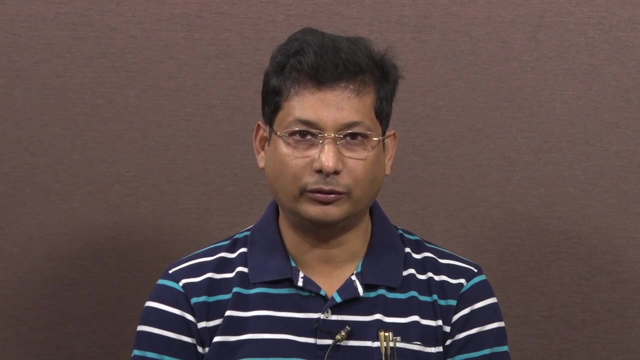 Welcome to NPTEL MOOC's course on Computer Vision and Image Processing: Fundamentals and Applications. I am Dr M K Bhunya, Professor of the Department of Electronics and Electrical Engineering, IIT Guwahati, So in this course I will discuss some fundamental concepts of computer vision. 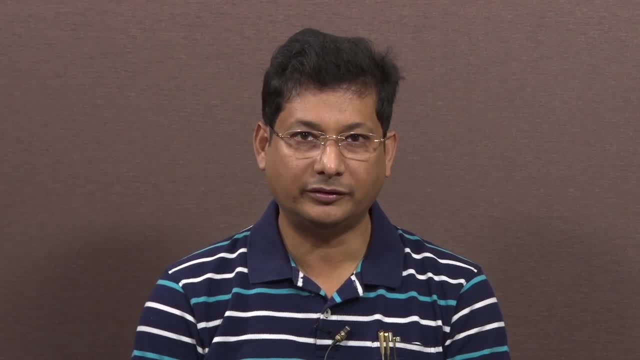 and image processing. And finally, I will highlight some important applications of computer vision. So what is computer vision? Computer vision is a field of computer science. The objective is to build a machine so that it can process and interpret images and the video. 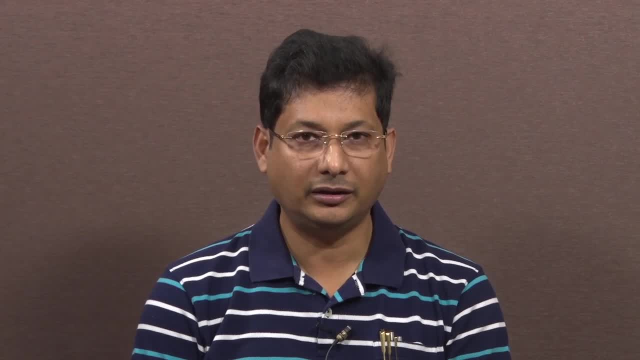 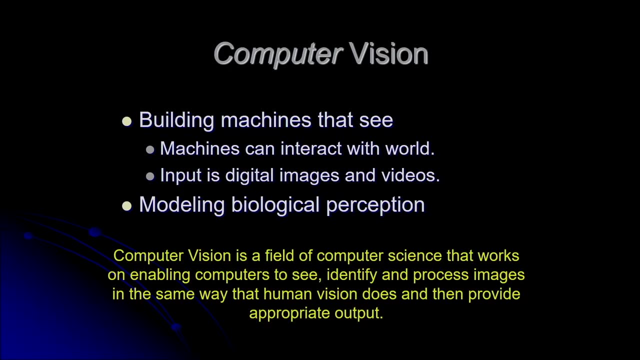 just like human visual system does. So I can say it may be a complement of biological vision. Let us see the formal definition of computer vision. So building machines that can see. Mainly the objective is to build a machine which can interact with world And 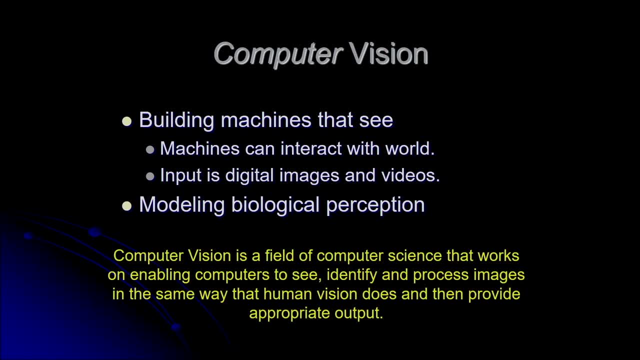 in a computer vision system, input is digital images and videos, and it is mainly the modeling of biological perception. So definition of computer vision is: computer vision is a field of computer science That works on enabling computers to see, identify and process images in the same way that human. 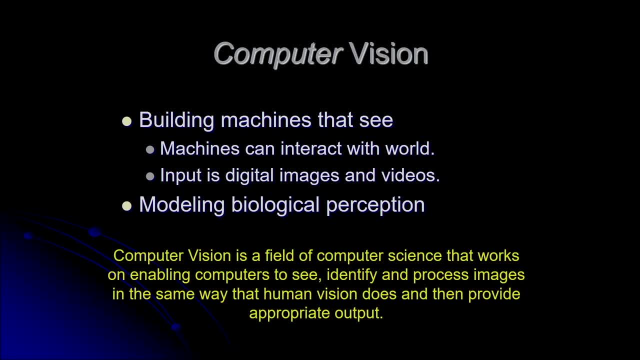 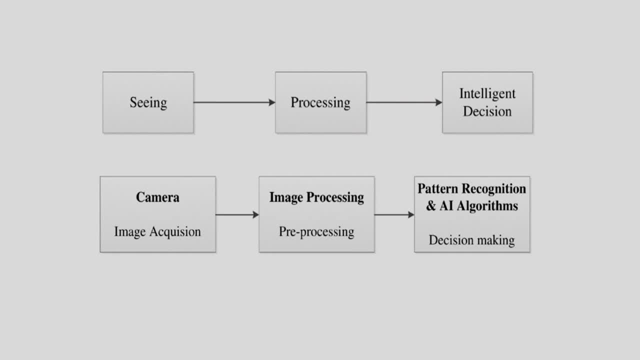 vision does and then provide appropriate output. So this is the definition of computer vision. In my next slide I want to show the similarity between the human visual system and the computer vision system. If you see the first block diagram, the first block diagram is the human. 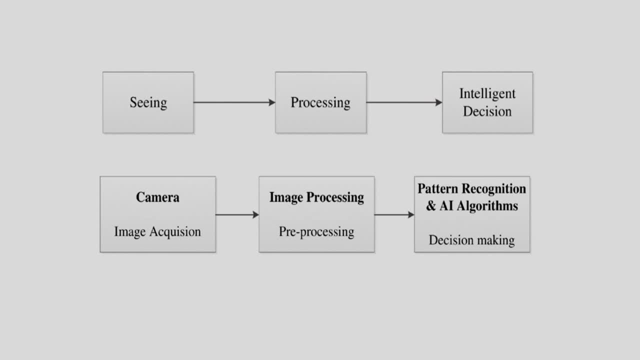 visual system. So, in case of the human visual system, we have eyes, We have eyes, We have eyes to see objects, or we can see images or we can see videos. After this we do some processing in our brain and after processing we take intelligent decisions. In case of 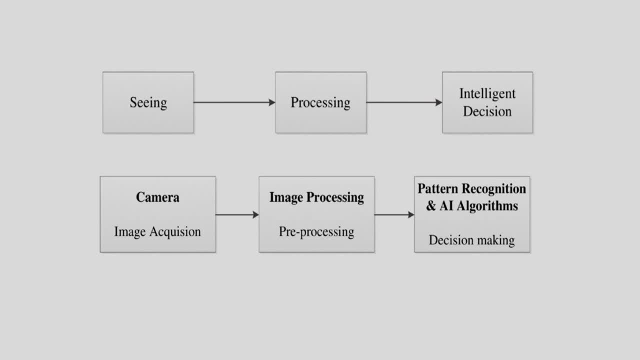 the computer vision system. we have cameras. We may have single camera or maybe multiple cameras for image acquisition, for video acquisition, And after this we do some processing, that is the pre-processing and that is called the image processing, And after this we have. 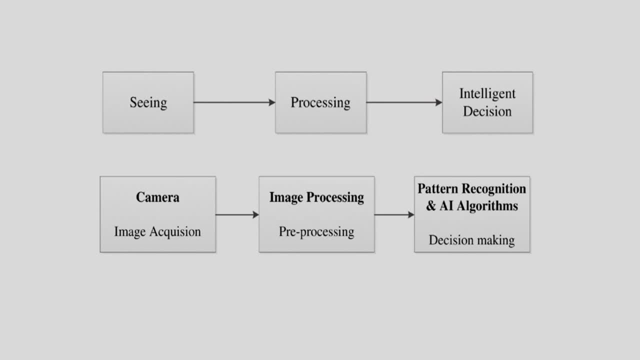 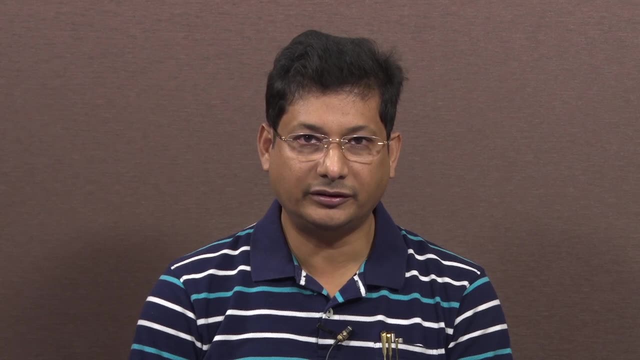 to apply some pattern recognition and artificial intelligence algorithms. So this is the intelligence algorithms for decision making. So in this case you have seen that the similarity between the human visual system and the computer vision system, In case of the human eye, the 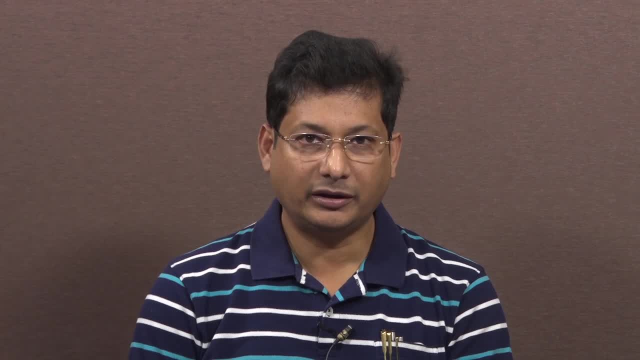 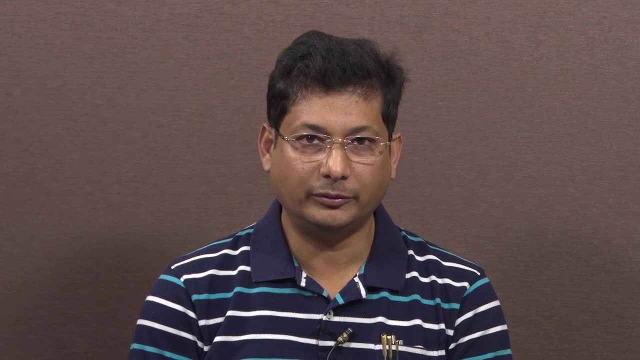 light photon is converted into electrical signal. In case of the camera, the light photon is also converted into electrical signal. So you can see the similarity between human visual system and the computer vision system. Now I want to highlight the distinction between computer vision, image processing and computer graphics. 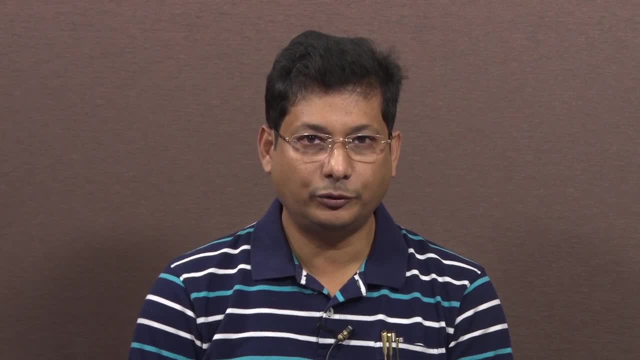 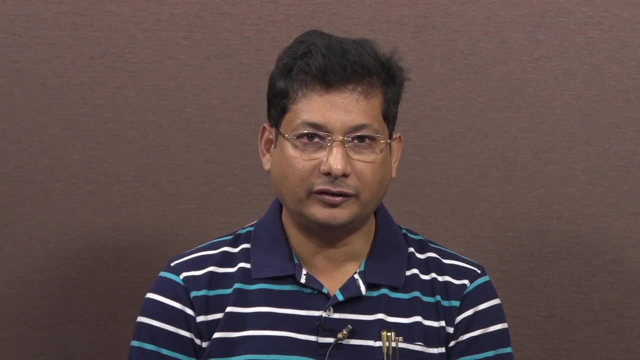 Assume that either a tree is harder, Everybody has experience with computer vision, So what I would suggest is all about much better data stabilization so you can get more information from a simple slide here. and I say that if in the online software there are intelligent 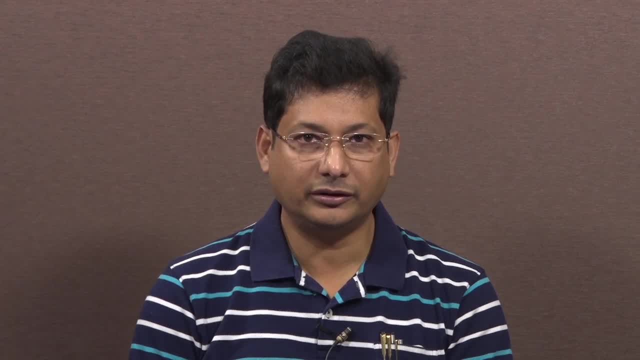 diskutations that you talk about and that is the opportunities that both computer vision and other electronic Pure Core method can offer. And, as in the mean time, or using our minute, Clark, 60 half times, which is applied to many, based on the performance of the computer. 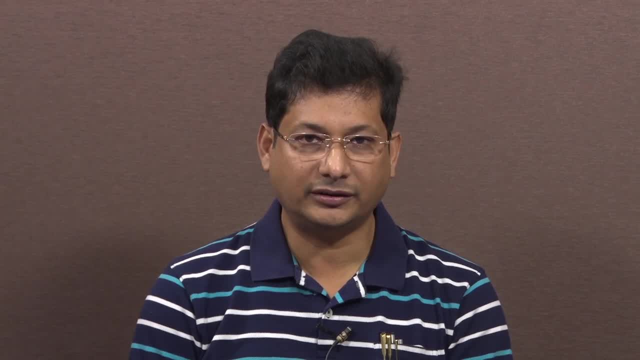 vision, my input is images or the videos and output is interpretations, The interpretation of images, interpretation of videos, that is computer vision. In case of the image processing, my input is image and output is also image. So I can give one example, Suppose, if I want. 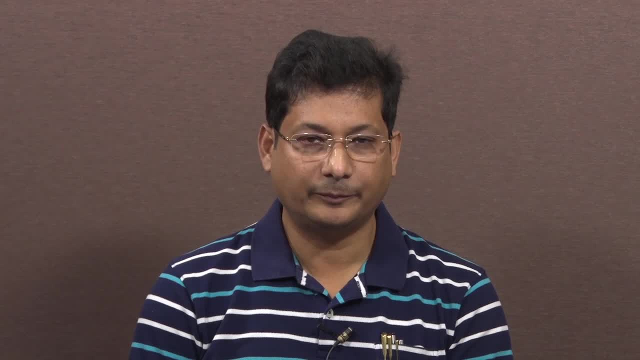 to improve the visual quality of an image, I have to do image processing. Then in this image, I have to do image processing. Then in this case my input is image, output is also image. In computer graphics my input is scene or the model. So from the model I have to generate the. 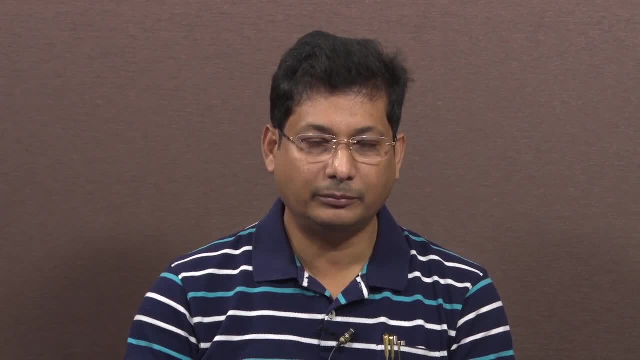 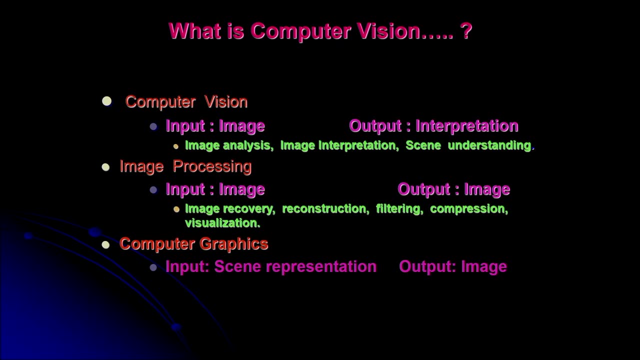 image. So in my next slide I want to show that distinction between computer vision, image processing and computer graphics. Here you have seen that computer vision is nothing but image analysis, image interpretations, scene understanding. So input is image, output is interpretation. 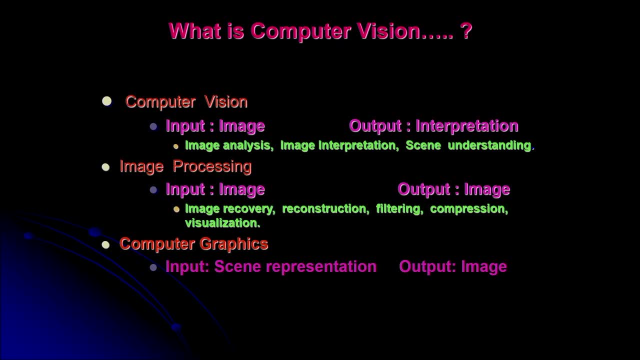 In image processing, input is image, output is also image. In computer graphics, input is model or scene and output is image. So that is the distinction between computer vision, image processing and computer graphics. Now let us see what are the applications of computer. 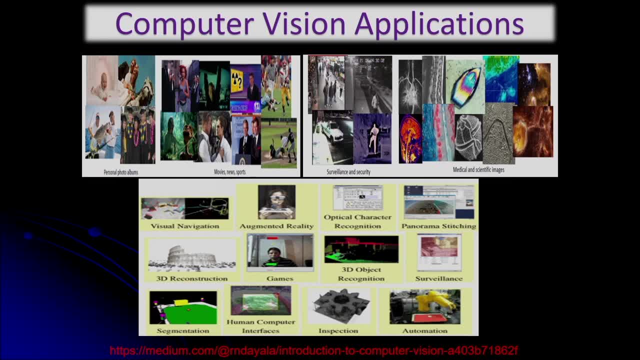 vision, the computer vision applications. So there are many applications of computer vision, like in multimedia video surveillance, in medical image analysis, medical image interpretations, and also like 3D reconstruction, image segmentation, human-computer interactions, 3D object recognition, optical character. 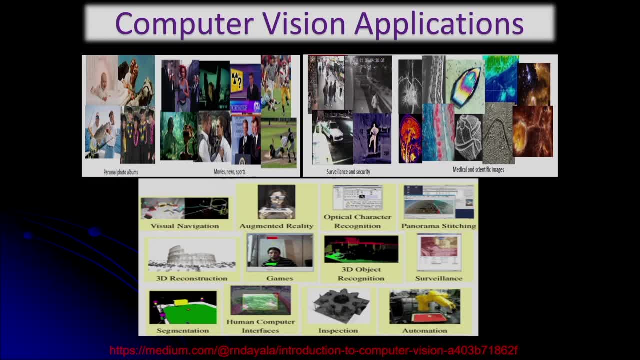 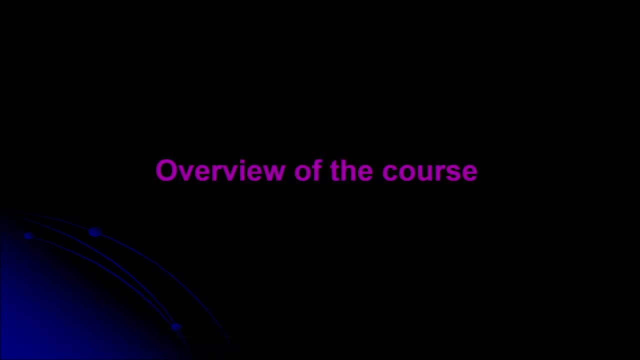 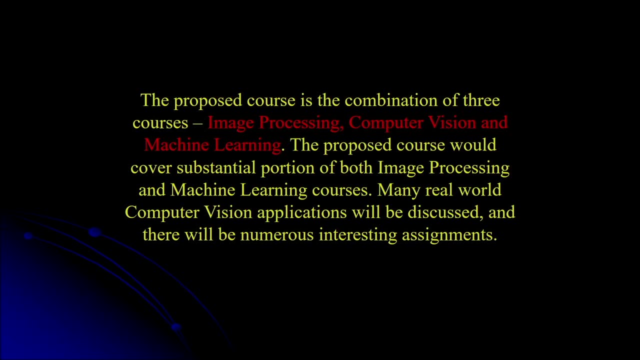 recognitions, augmented realities, video surveillance, inspection of industrial components and automation. So there are many, many applications of computer vision. Now, overview of the course. The proposed course is the combination of three courses, mainly the image processing, computer vision and machine learning. The machine learning: 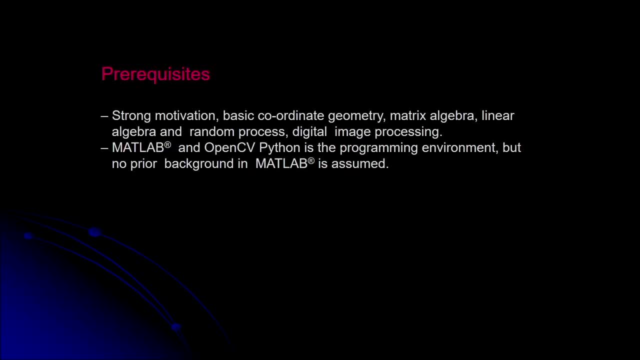 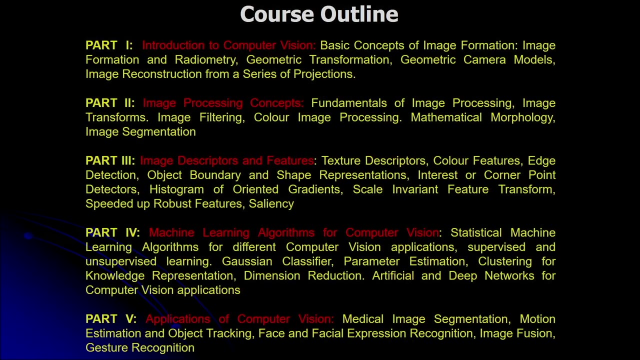 algorithms used in computer vision applications. The prerequisites: the basic coordinate geometry, matrix algebra, linear algebra and random process, digital image processing. And for programming we can consider MATLAB or maybe OpenCP, Python. Now let us see the course outline. 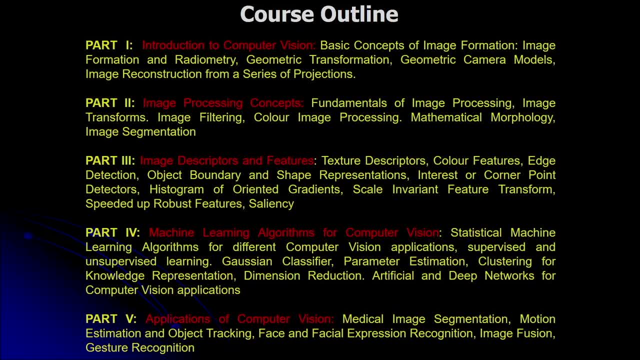 The part one is introduction to computer vision. So in this part I will discuss the basic concept of image formation. image formation and the radiometry, geometric transformation, geometric camera models and image reconstruction from a series of projections. So part two is the image processing concepts. So in this case we will discuss the fundamentals. 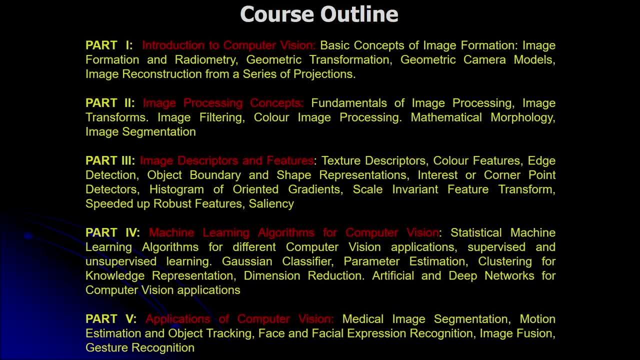 of image processing, image transform, image filtering, color image processing and also mathematical morphology and image segmentation. Part three is image descriptors and features. So in this case we will discuss the texture descriptors, color features, edge detection, shape representations and some features like hawk features, sheep features. 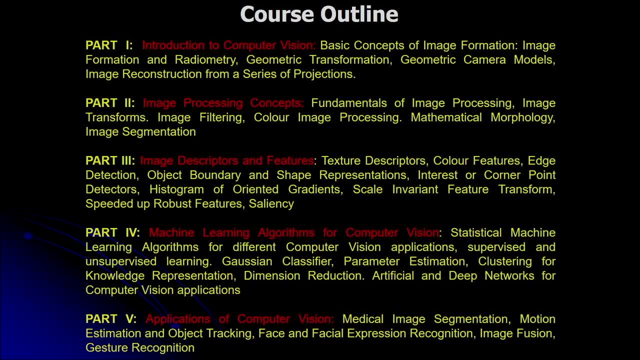 shark features and the concept of saliency. we will discuss And after this the machine learning algorithms for computer vision. So we will discuss the supervised algorithms and the unsupervised algorithms for machine learning algorithms for computer vision. Also, we will discuss artificial neural networks and deep networks. 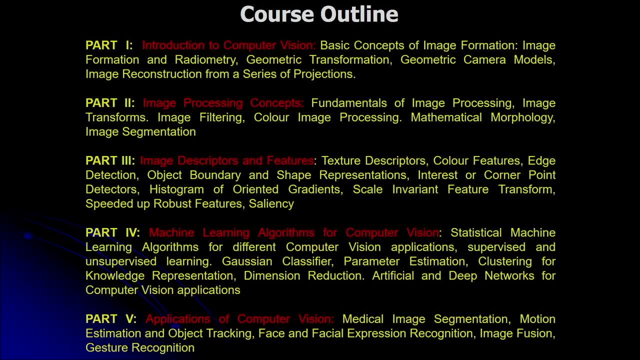 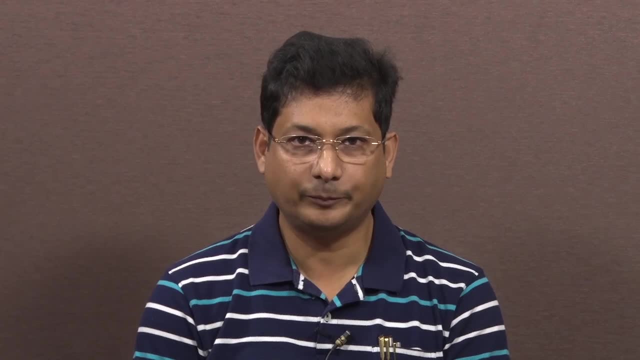 And finally the applications of computer visions. So we will discuss medical image segmentations, motion estimation and object tracking and face and facial expression recognition, image fusion and gesture recognitions. So we have seen that in this course. first part is the concept of image formation, camera model and radiometry.